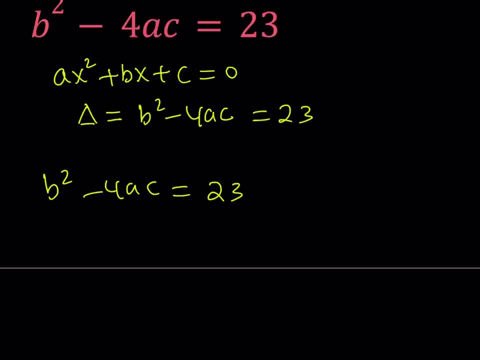 we use in number theory. So if you look at this equation carefully, you're going to notice that 4 times ac is a multiple of 4. therefore it's always even. So this is an even number. We also know that b squared minus an even number is 23, which is an odd number. So when do you get an? 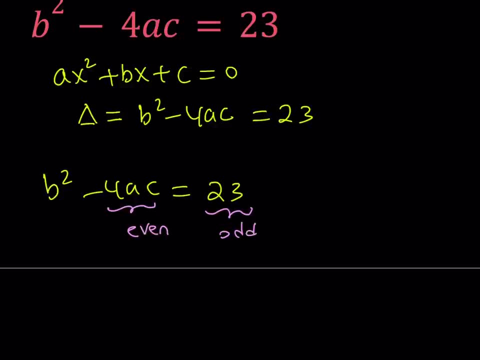 odd number. If you subtract an even number from another number, that number also needs to be odd. So in other words, odd minus even is equal to odd. Otherwise, if you subtract even number from an even number, the difference is also even, And you can easily prove this. That's very easy to prove. 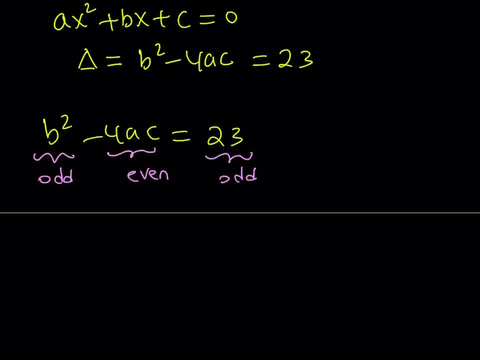 Now what does that mean for b squared to be odd? If b squared is odd, it implies that b is odd. Right Simple. Because if a number is not odd, like, even its square cannot be odd either. So we can prove by- you know- contradiction that this is impossible. 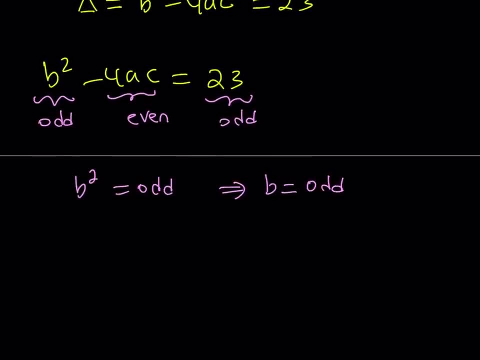 Okay, so b needs to be odd as well, and that implies a very important result, And this is actually the breaking point for this problem. So since b is odd, I can replace b with 2n plus 1, where n is an integer, So n is an integer. 2n plus 1 represents an odd number. So if b is odd, 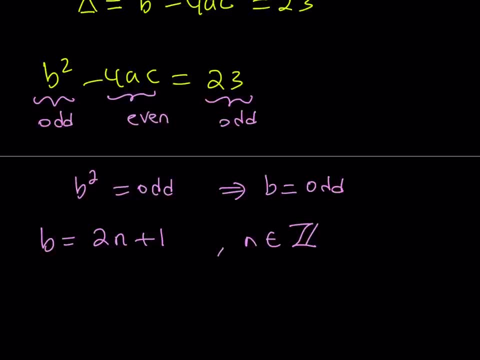 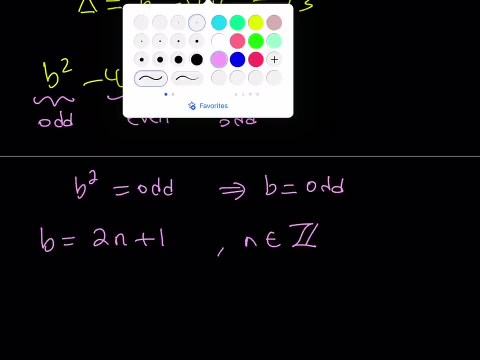 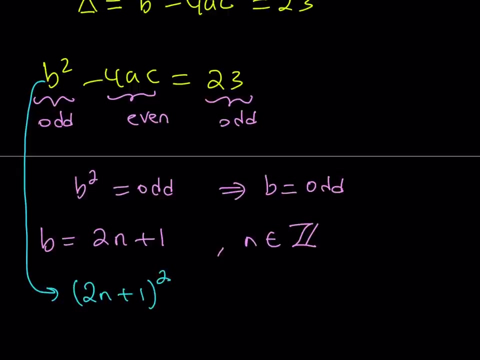 number and we're going to substitute this. as you know, substitute substitution is a very important rule. It plays a very important role in solving very many problems. Okay, let's take a look. So I'm going to replace b with 2n plus 1 here. That gives me 2n plus 1, quantity squared minus 4ac. 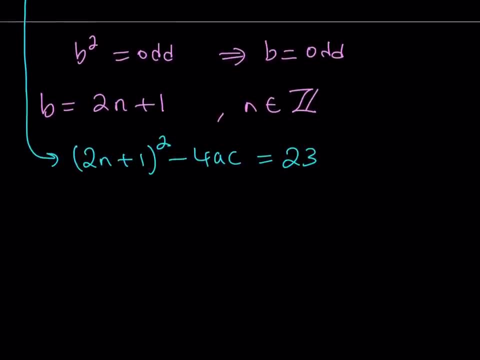 equals 23.. And again, n is an integer, a is an integer, c is an integer. So here everything, every variable, represents an integer. Let's go ahead and expand 2n plus 1.. It is 4n squared plus 4n plus 1 minus 4ac equals 23.. 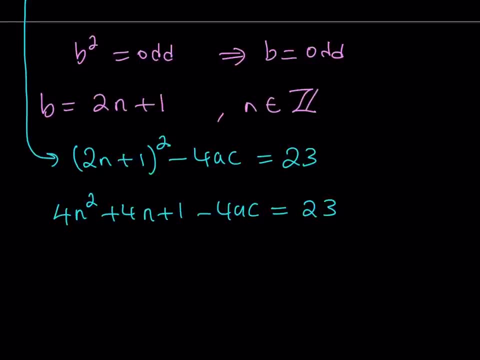 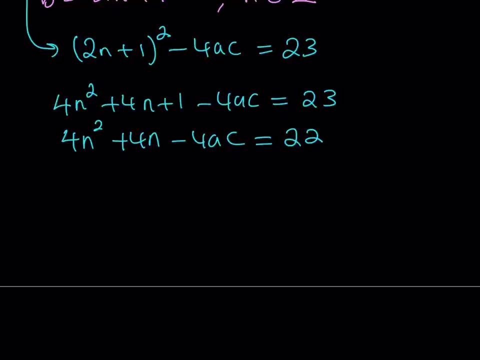 Now it will be meaningful to subtract 1 from both sides, so that we can have a number on the other side and all the variables on the left hand side. Great, And this gives us 22.. Now this is super duper important from a number theory perspective, because if you look at the left hand side, you can 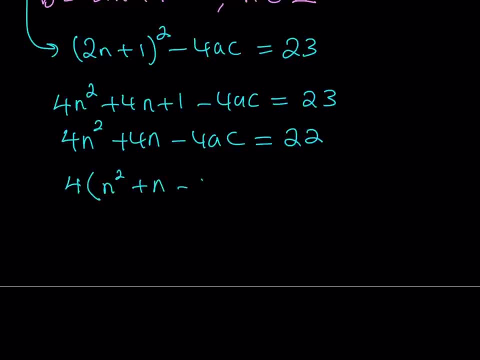 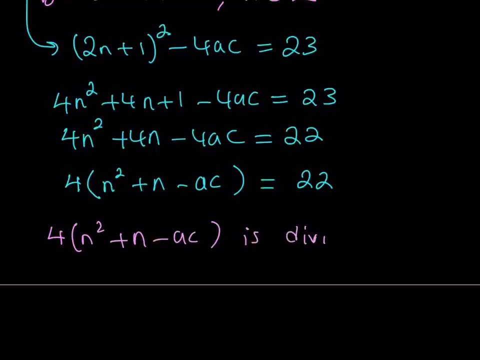 factor the 4 out. And what is that supposed to mean? It means that the expression on the left hand side is a multiple of 4.. Which means that this expression on the left hand side is divisible by 4.. So our conclusion here is: 4 times the quantity n squared plus n, minus ac is divisible by 4 because it is a multiple. 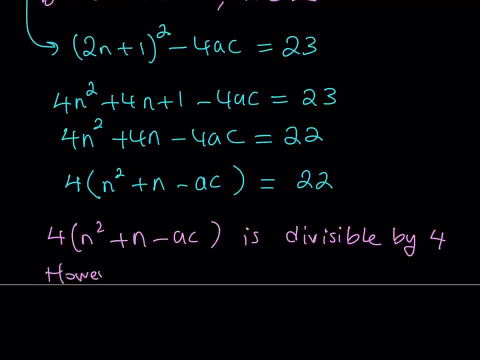 of 4.. Makes sense, right? However, 22 is not divisible by 4, as we well know, right? Because 24 is a multiple of 4,, 20 is a multiple of 4, 22 is in between. it is not divisible by 4.. 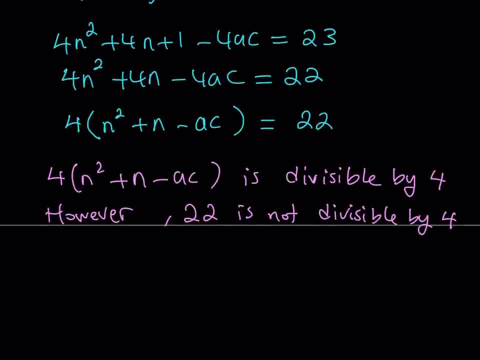 So you get a remainder when you divide 22 by 4. obviously, What is that supposed to mean? It means that hence we can write it in mathematical words: That is a very mathematical word, right? There are no integer numbers solutions. Why? Because you got an equation where the left-hand side is divisible by 4,. 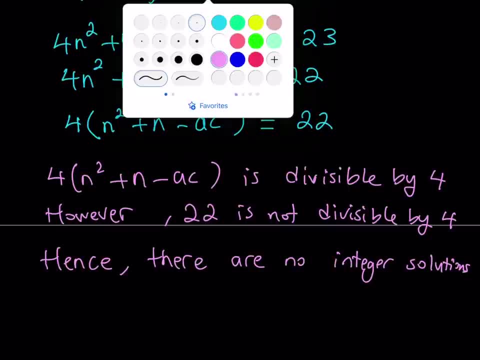 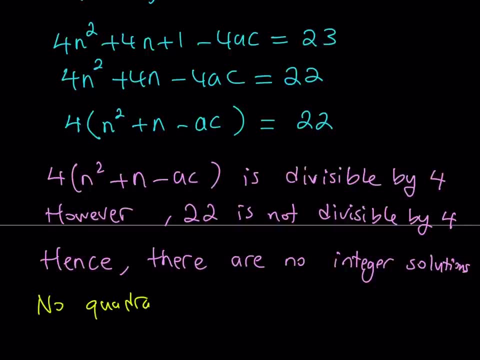 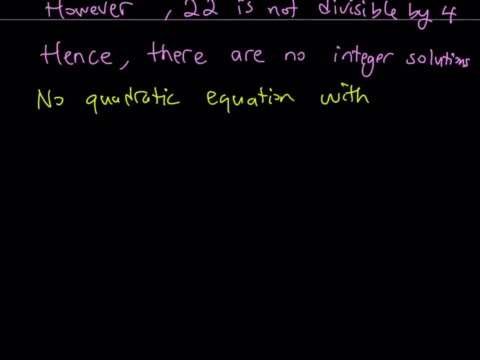 but the right-hand side is not divisible by 4, and this is impossible. Therefore, we have no quadratic equation, no quadratic equation with integer coefficients. with integer coefficients- oopsies, I'm going to mess up on the word having 23 as its discriminant. 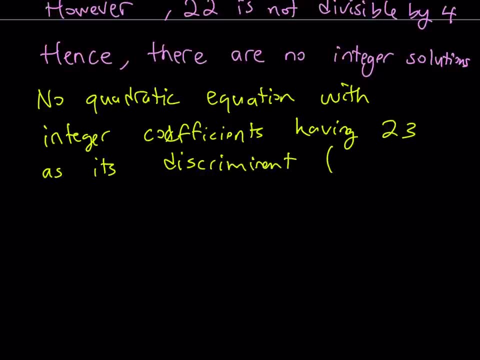 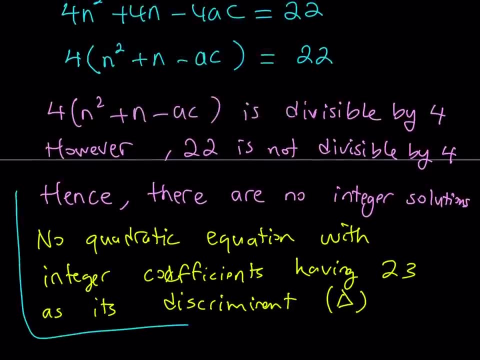 which is delta right. And that is going to be our conclusion, And this brings us to the end of this video. Well, thank you for watching. I hope you enjoyed it. Please let me know. Don't forget to comment, like and subscribe. I'll see you tomorrow with another video. Until then, be safe. take care and bye-bye.